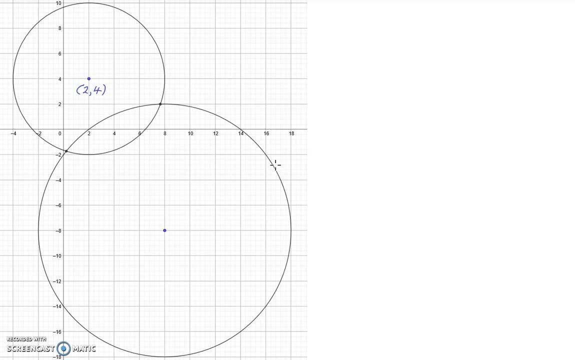 So the equation for the smaller circle is going to be: x minus 2 squared plus y minus 4 squared equals the radius, which is 6 squared 36.. I am now going to expand these brackets. I am going to use the bits to give. 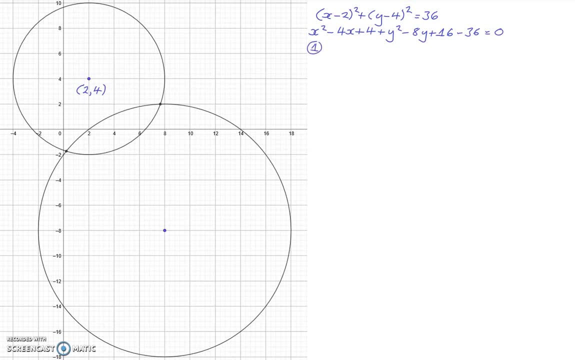 and simplifying that and denoting the simplified equation as equation 1.. 1 gives this. And now, similarly, looking at the larger circle whose center has coordinates of 8 minus 8.. And the radius is going to be from 8 to minus 2.. 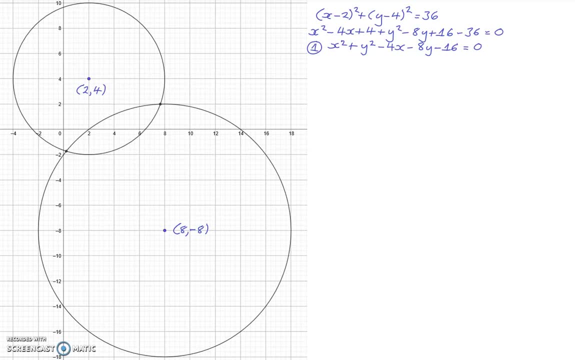 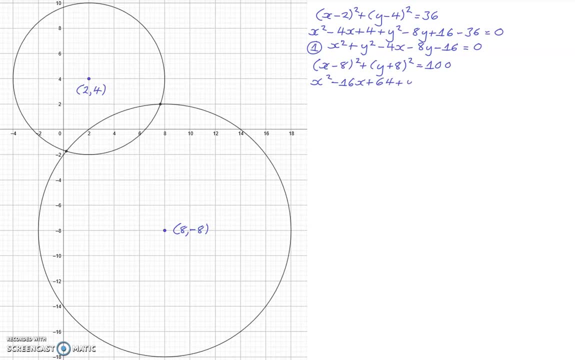 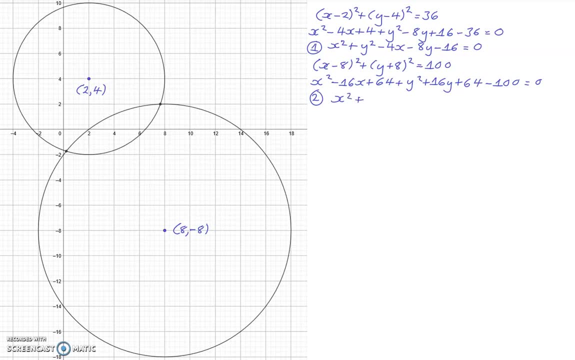 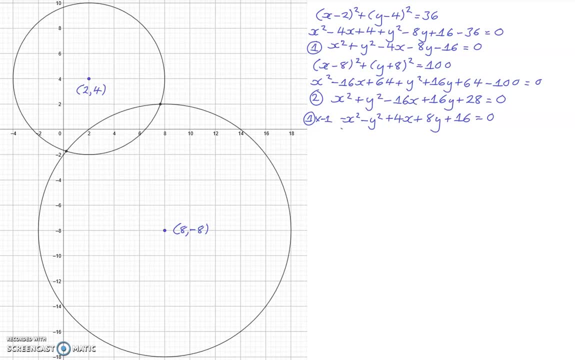 Now we add these two equations together, now Which gives? Now, if you rearrange that to make x the subject, this gives x equals. Now I'm going to substitute this into equation 1.. So sub into equation 1. And this will give. 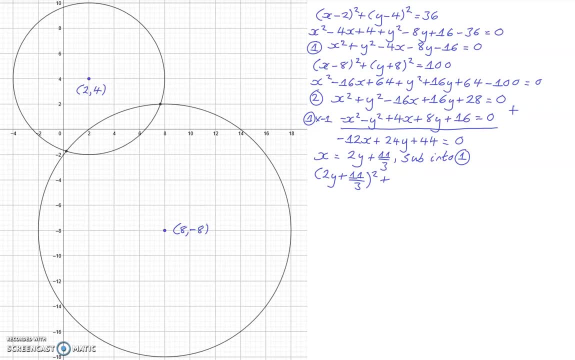 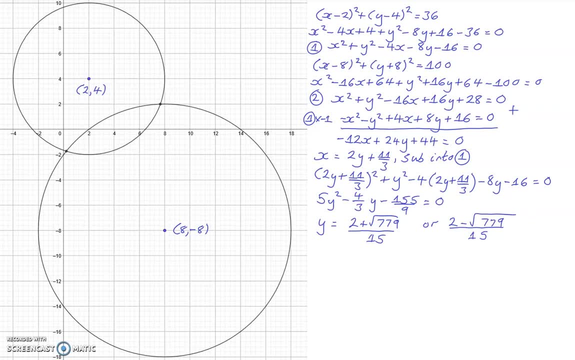 The next thing to do is to find the X coordinates for each Y value. So X equals. So we're going to use this Equation here to find the corresponding X values. So we're going to have two, And then the Y coordinate. 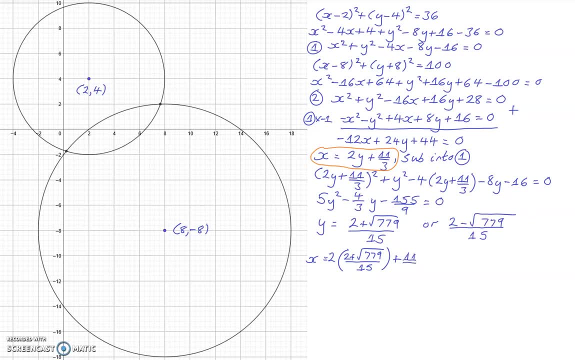 Plus 11 over three. So that gives the X X coordinate exactly as, And similarly for the other Y coordinate If that's corresponding X coordinate as. So the exact coordinates of the two points intersection are as shown. So this Point is. 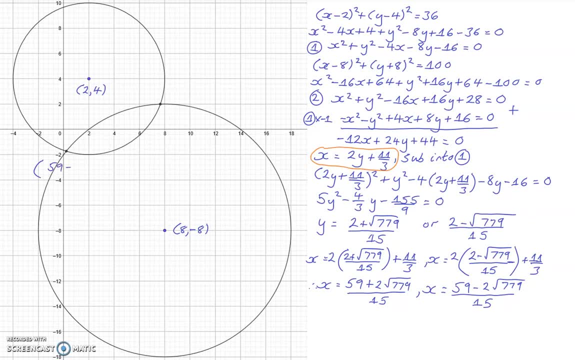 One: Find the definite relationship of The X coordinate to the Y coordinate of the two. Now, Here we go. And this iko: OK, Let's look at that. So Point is Now, if you convert these coordinates to decimals, to three decimal places, we have this: 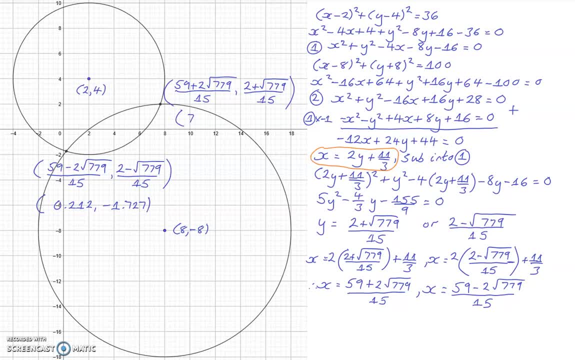 And for this point, And I'll put the actual grid onto the axes so you can see that the white one of this point, here, the upper point, is well, almost two. So one point nine nine four checks out the X coordinate. This slot is around. 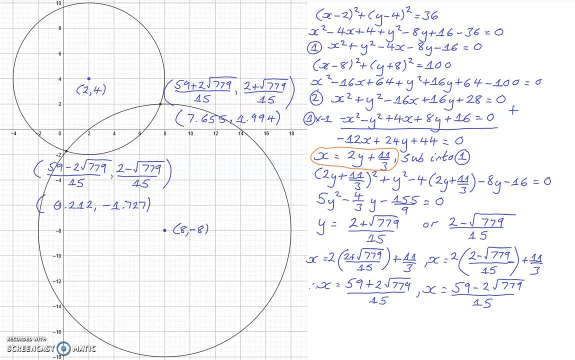 Seven point six. Well, that's correct as well. The X coordinate of the lower point, zero point two, because each little square on the X and Y axis is equivalent to zero point four units. So that's probably that's that point. Now the X coordinate is about half a square. 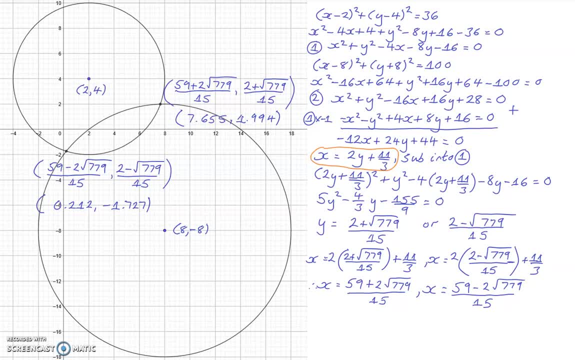 So half of zero point four, zero point two, And similarly the Y coordinate Is halfway between minus one point six and one and minus one point six and minus two, So about minus one point eight, Again very close. So the coordinates I found are indeed correct. Hope you have found this video useful.